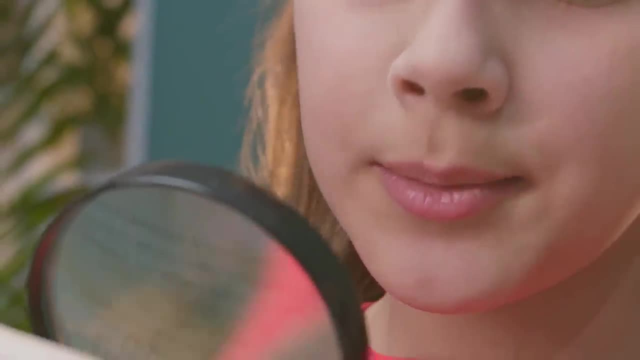 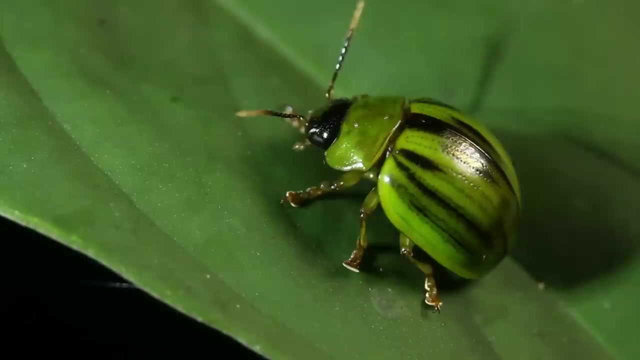 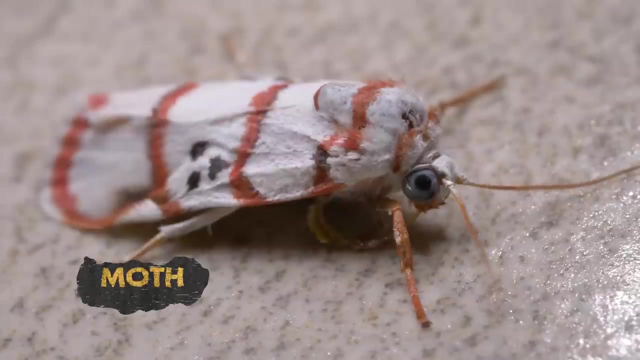 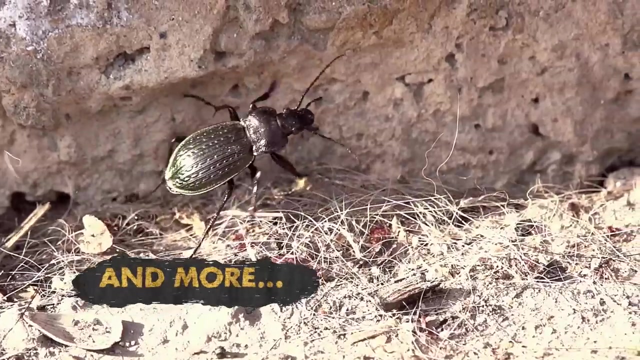 interested in. Let's take a look at some of the things that insects have in common. First, their bodies are made up of three sections: a head, thorax and abdomen. Birds, moths, butterflies, ants, mosquitoes, bees and other insects have the same three. 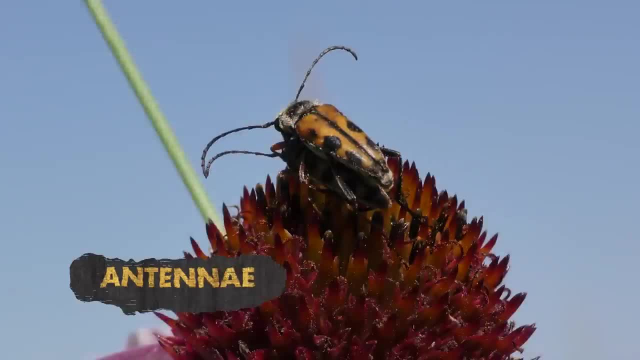 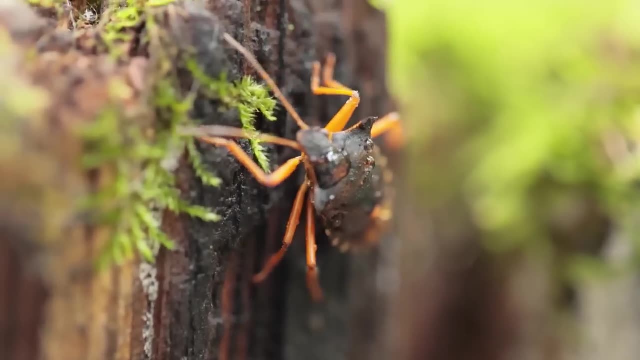 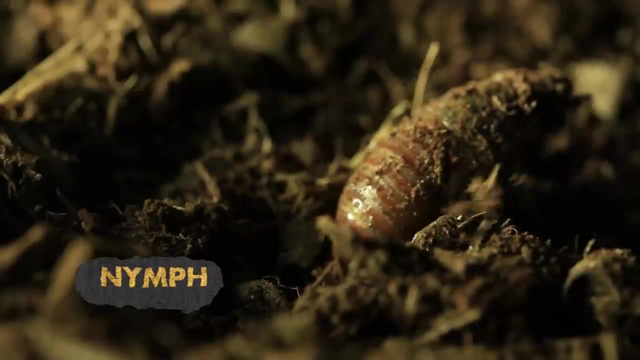 sections. Second, all insects have a pair of antennae on their head and six legs attached to their thorax. Third, all insects are born from eggs. The young or baby insects are called nymphs. Nymphs are born from eggs. Nymphs are born from eggs. Nymphs are born from eggs. Nymphs are born. 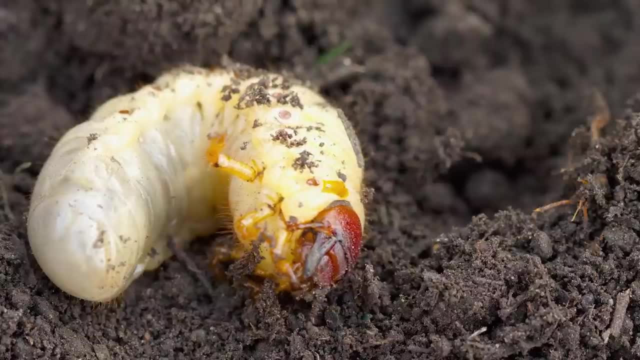 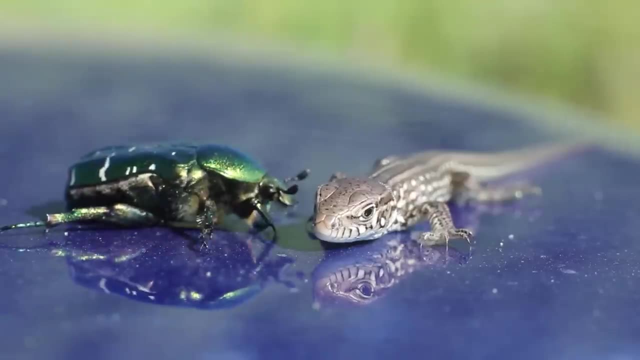 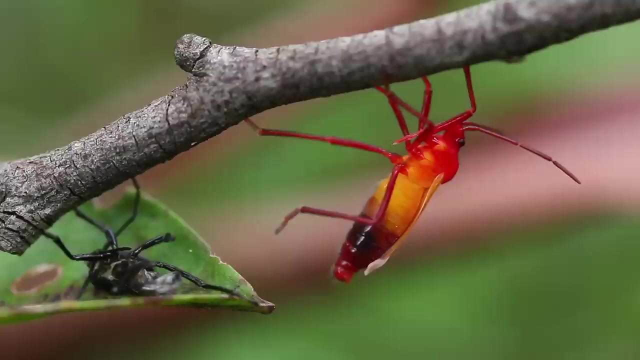 with an outer covering, which is replaced after birth by something called chitin. Chitin is an insect's exoskeleton. It is a strong material that helps protect the insect. This growth process is called molting. Molting happens when an insect becomes too big for its 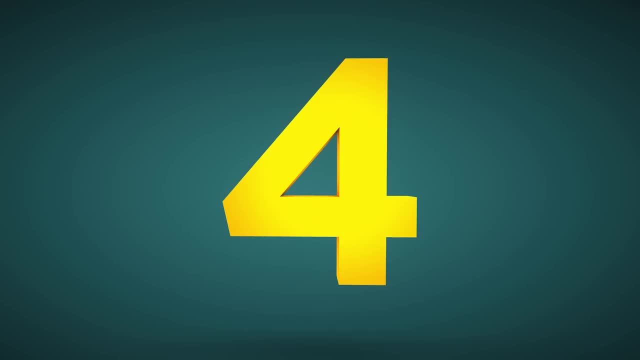 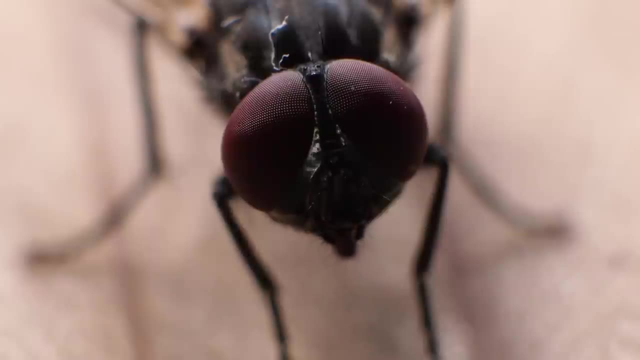 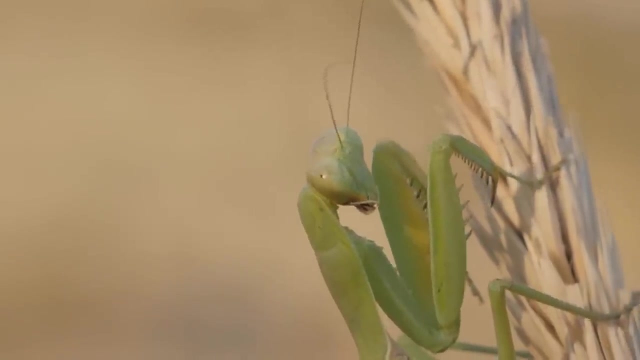 exoskeleton, so it sheds it. Fourth, insects have specialized eyes called compound eyes. Their eyes help them see things all around them, not just in front. like your eyes, They also can see things that move very quickly. Fifth, some insects can fly and their wings are connected. 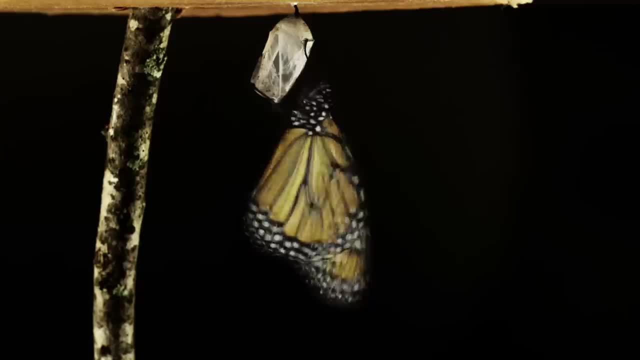 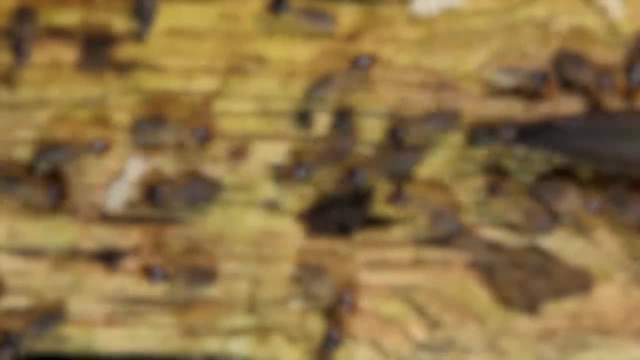 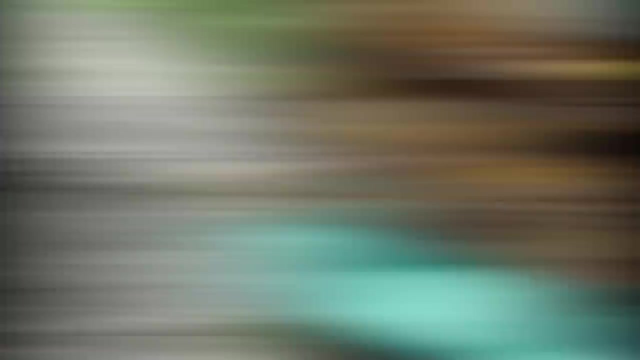 to their thorax. There are several categories of insects. One is called social insects. A social insect is an insect that lives in colonies with a lot of other insects. One is called social insects insects of the same type. Bees, ants, termites and wasps are all social insects. 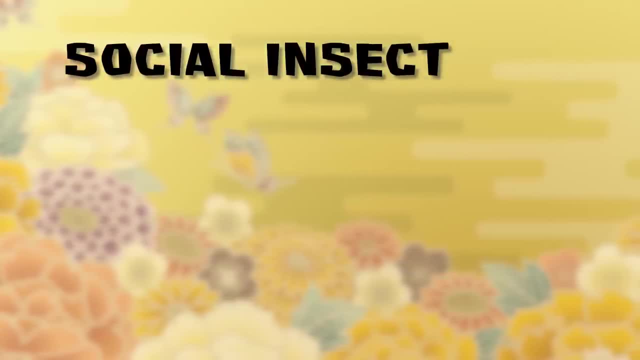 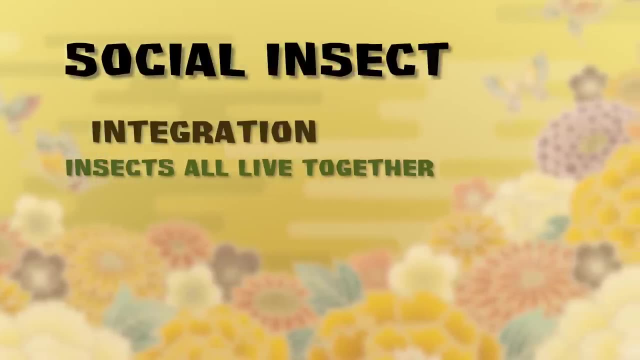 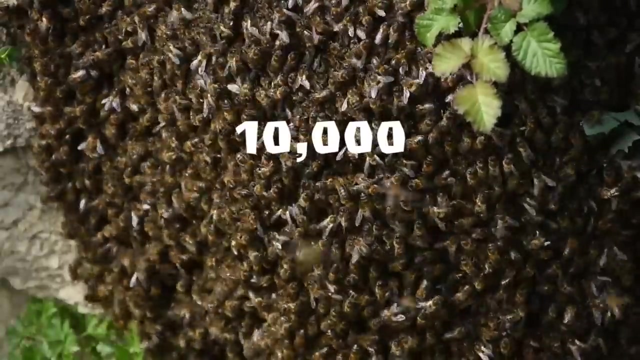 To be a social insect, you must fit into the following three groups. The first is called integration, which simply means that insects all live together. A beehive is one example of this. There can be anywhere from 10,000 to more than 60,000 bees in 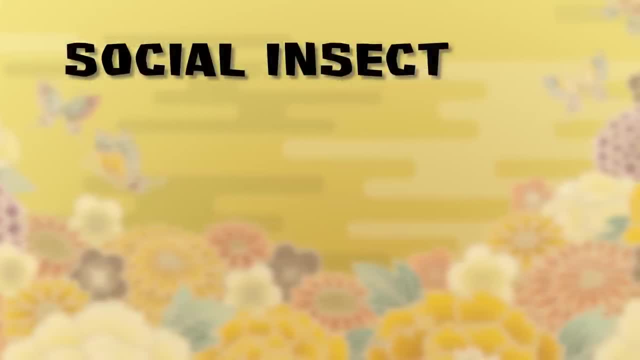 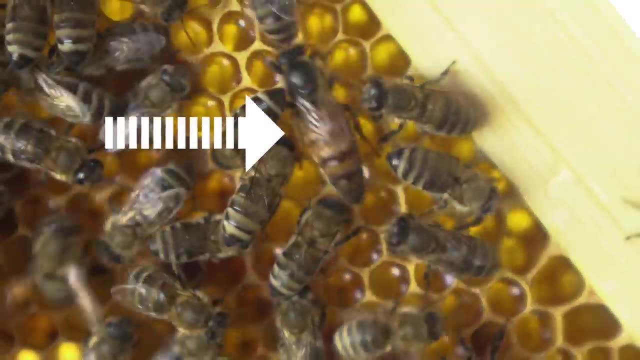 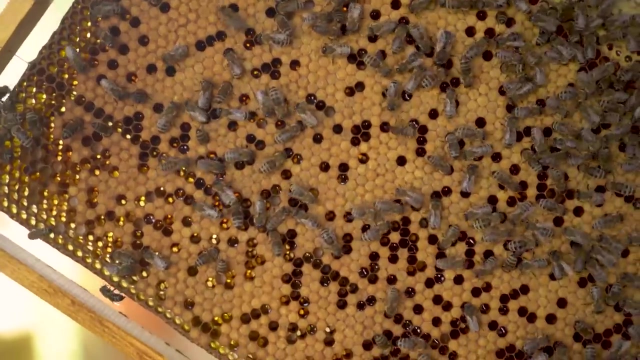 one hive. Another group is called division of labor, which means they each have a special job to do. A queen bee lives for several years. One of her jobs is to lay a lot of eggs. A queen bee can lay around 2,000 eggs a day. 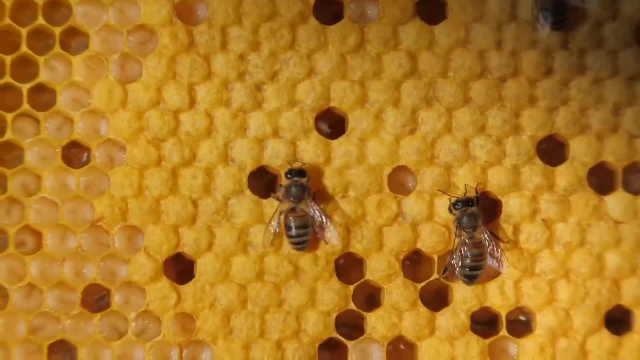 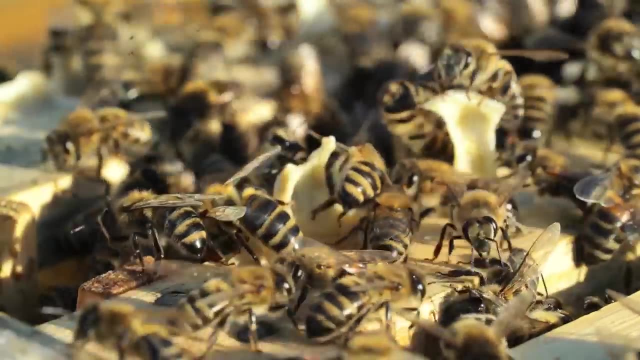 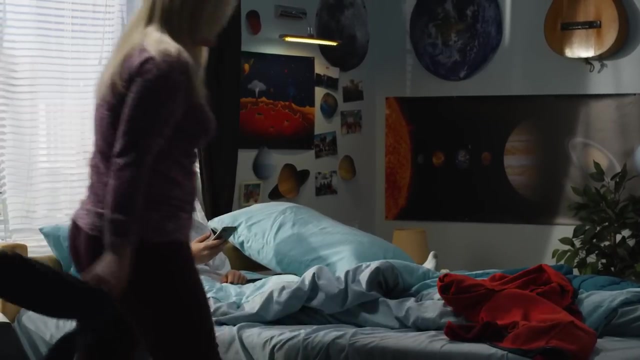 That's a lot of eggs to make in a single day. She also produces a special scent. When the worker bees can smell her scent, they know she is near and they continue working. Do you ever find yourself getting sidetracked from a job that your mom might have given you? 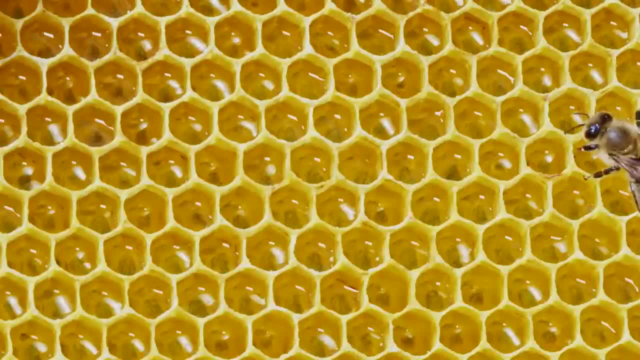 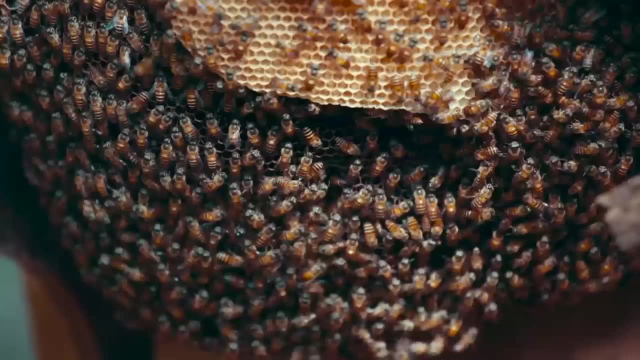 if she isn't right next to you. Well, when the queen gives off her special scent, the worker bees know she is home and they keep working. But if they don't see her, they don't know she is home. But if they don't see her, they don't know she is home. 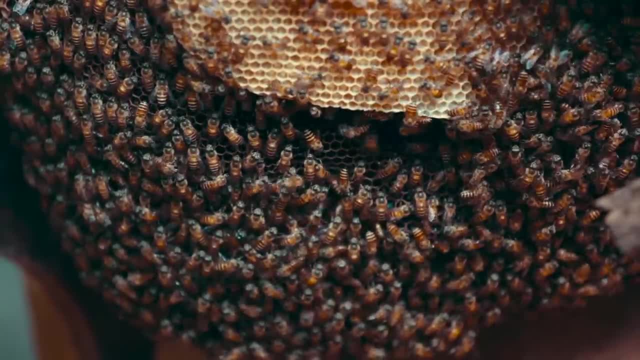 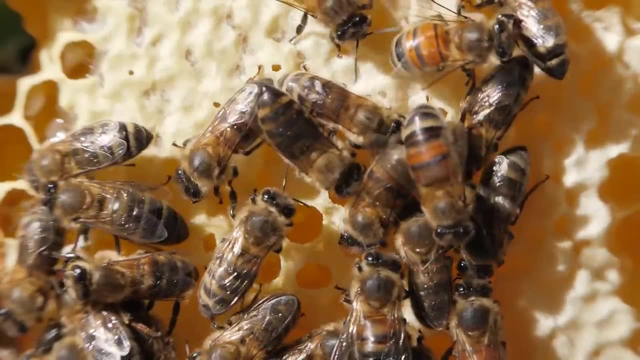 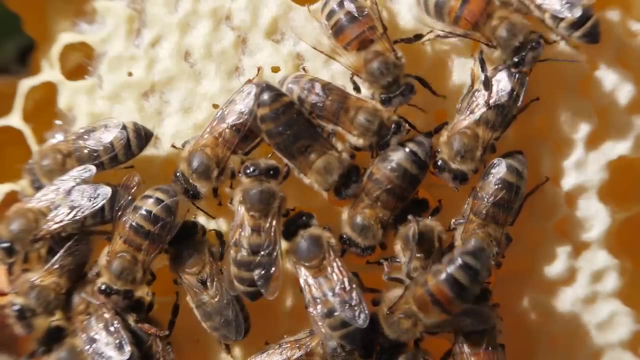 When they smell her, they think she is gone, And then they think they need to start laying the eggs. This isn't their job, it's hers. So to keep them focused, the queen releases a smell that reminds them that she is home and to keep doing their jobs. 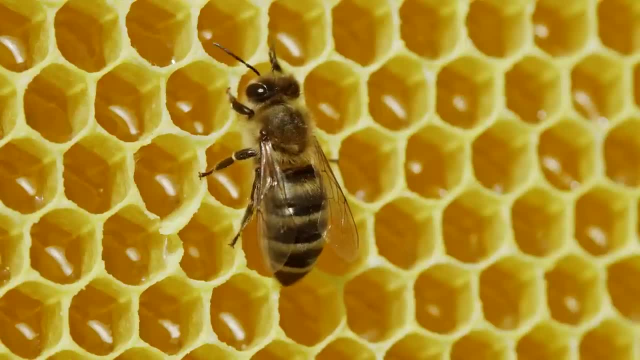 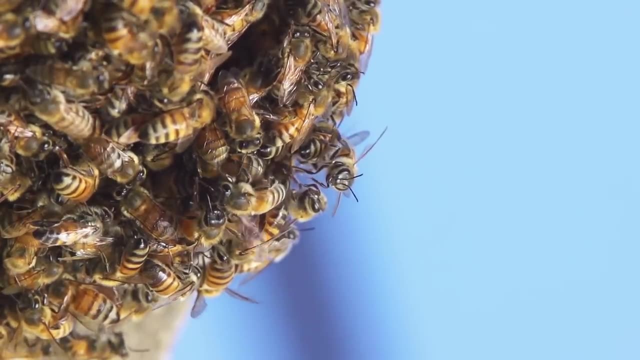 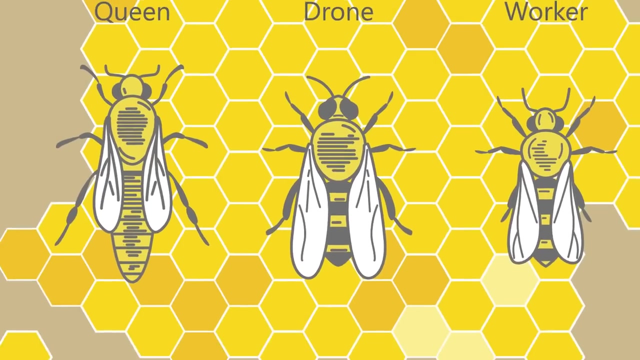 The worker bees are all female. They live for only a few short months. Their job is to feed the queen, collect pollen and nectar, make beeswax, keep the hive clean and defend it. The male bees are called drones. Their job is to mate with the queen. 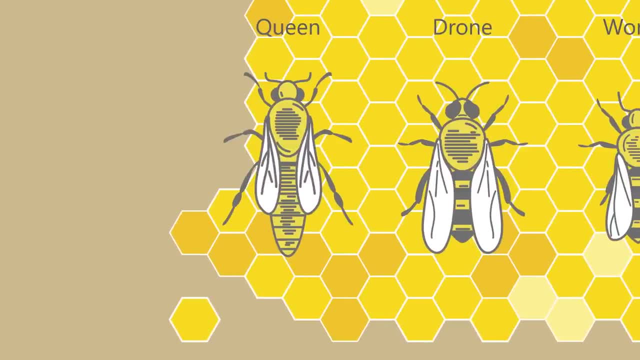 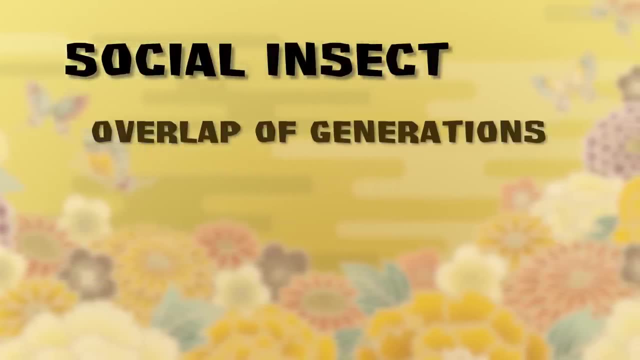 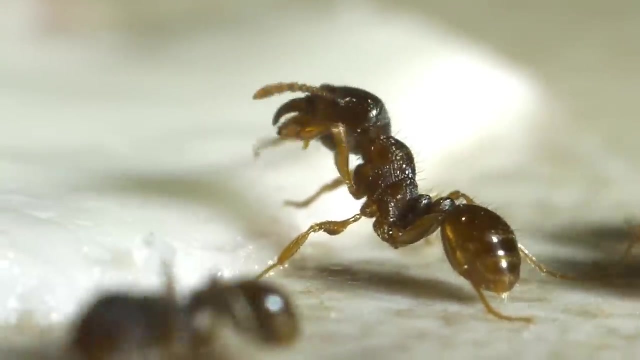 so she can lay the eggs that make more baby bees. The third group of social insects is called overlap of generations. That simply means both young and old live in the colonies together. Many insects live on their own, but social insects live in the colonies. 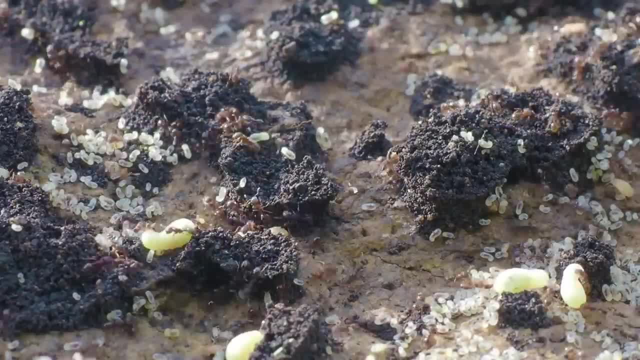 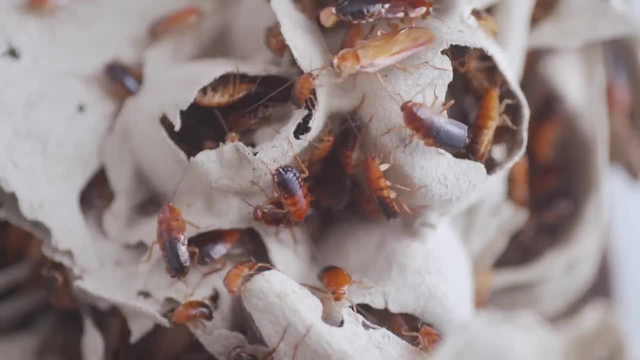 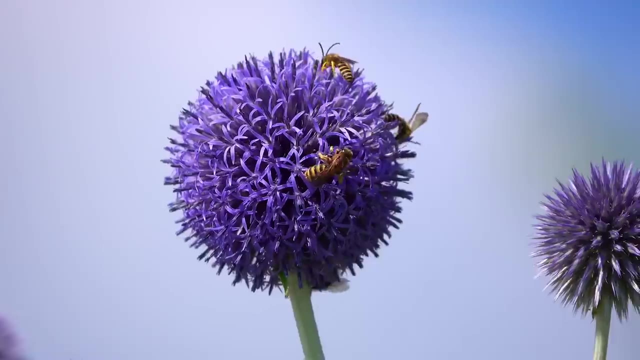 They live and work together in large groups. They do this to build homes as well as to help them survive. But insects don't just ensure their own survival. they help us. too. Many are beneficial to the environment in several ways. Bees can deliver good bacteria to plants. 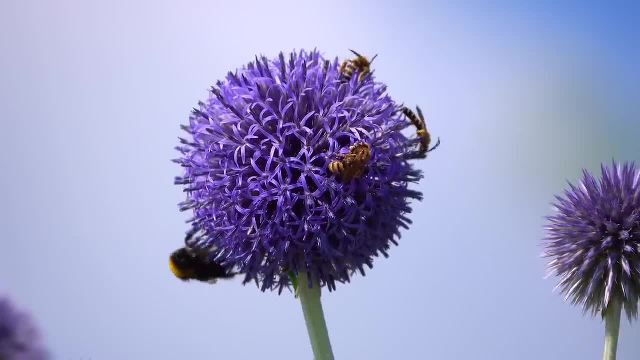 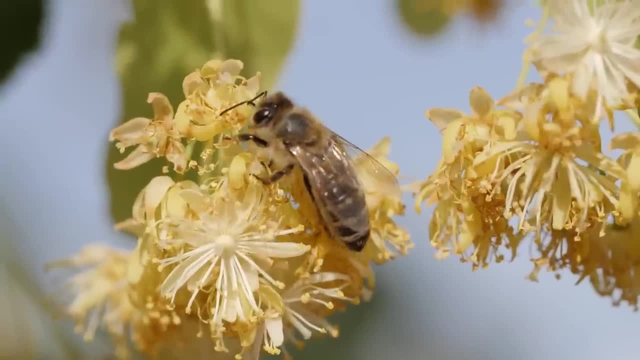 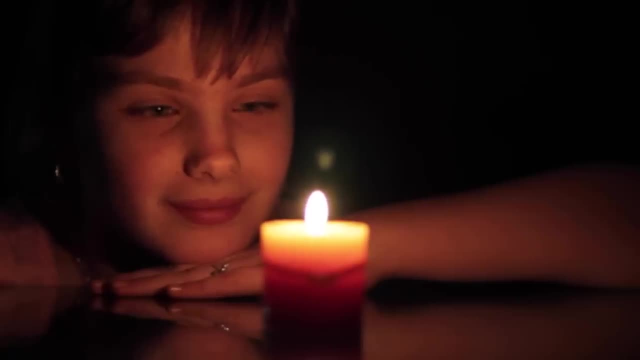 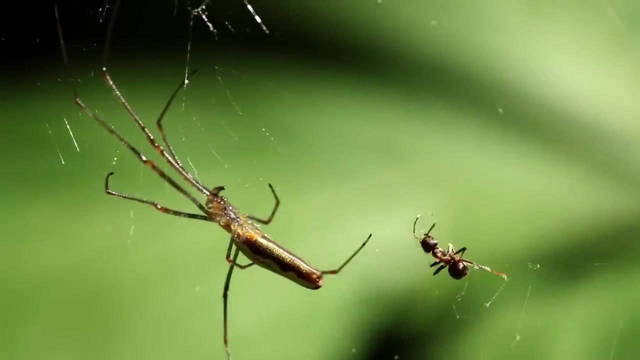 and spread seeds. Bees can also pollinate flowers and spread seeds, Which helps more flowers and plants grow. They produce delicious honey for you to eat, as well as wax for candles. Most bugs are part of the arthropod family, which includes insects and spiders. 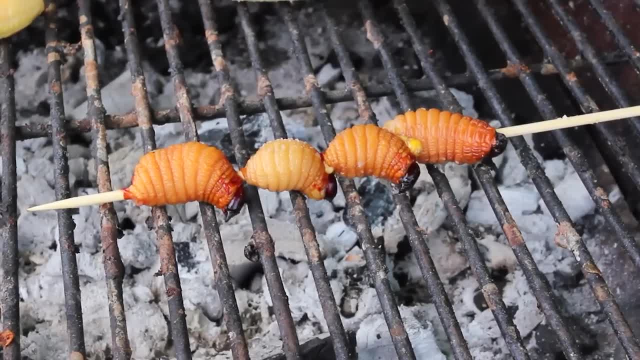 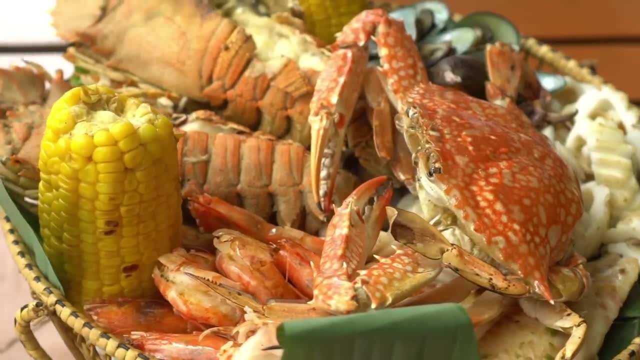 Do you think it's gross to eat a bug? Well, some people pay a lot of money at a fancy restaurant to eat one. Many people might not realize that they're eating a bug, But they're not. If you have a bug, you're eating a bug. 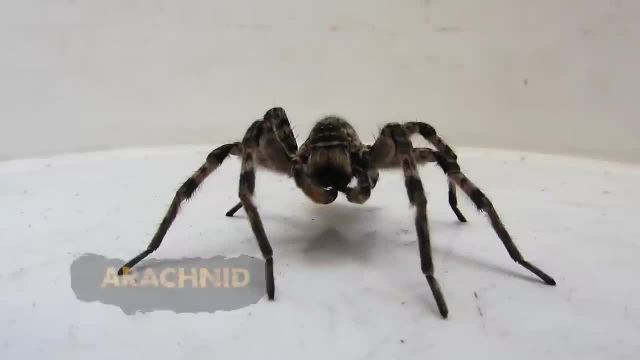 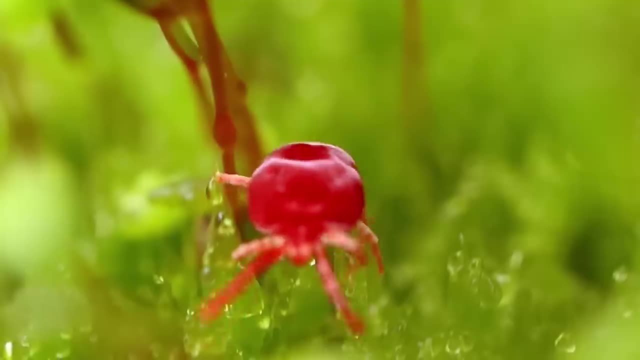 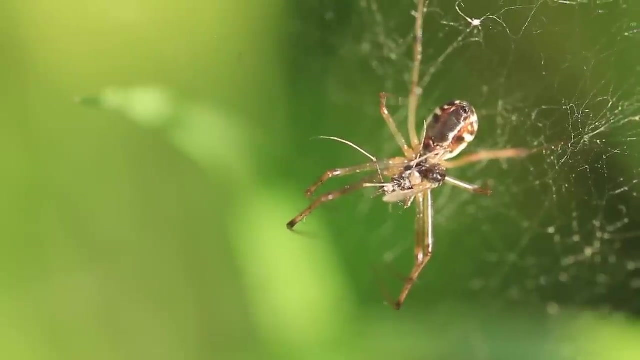 The most harmful bugs are the ones that attack your body. Spiders are part of a group called arachnids. Arachnids also include scorpions, mites and ticks. Unlike insects with three body parts, arachnids only have two main body sections called. 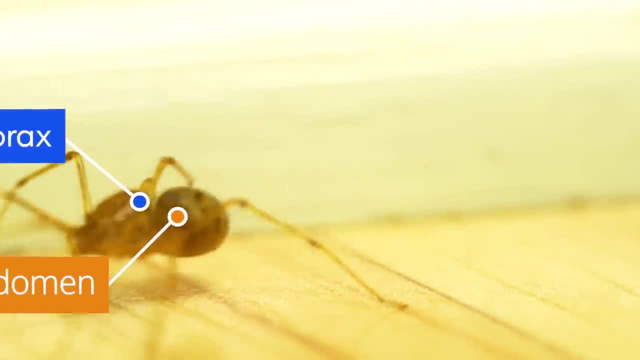 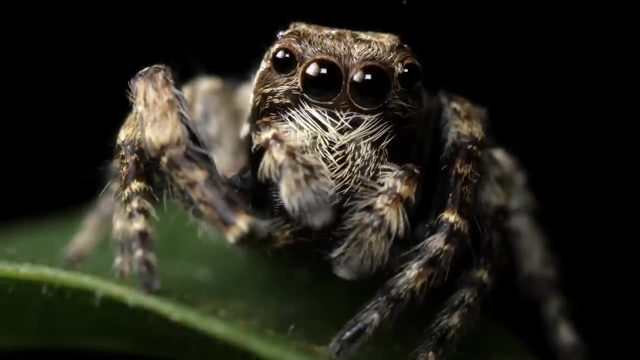 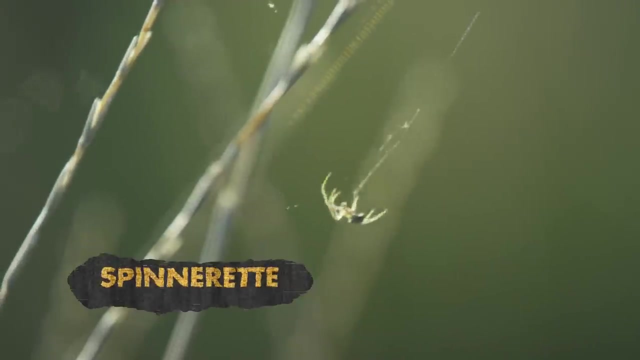 the cephalothorax and the abdomen. Arachnids have eight legs, which is two more than the abdomen. Arachnids have four eyes, which are smaller than an insect, and simple eyes instead of compound eyes. They do not have antennae or wings either. Spiders' bodies have something called a spinneret. 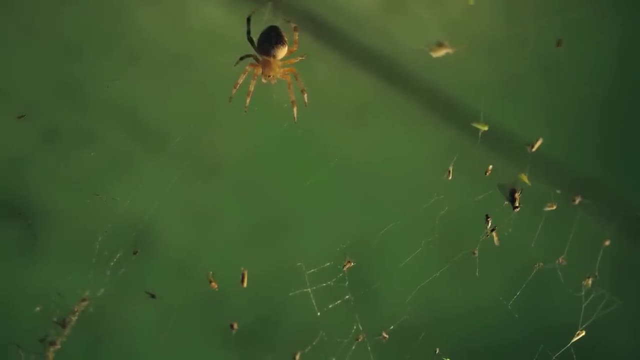 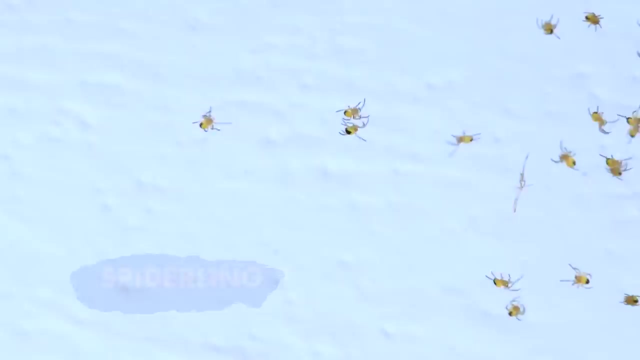 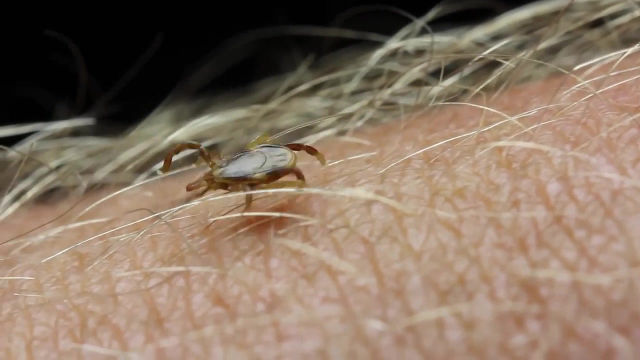 which produces silk. They use the silk to spin their webs and to catch their prey. Female spiders make cocoons out of their silk to hold and protect their eggs. When those eggs hatch, the young spiders are called spiderlings. Some arachnids and insects, like ticks, can cause harm to humans and other mammals. 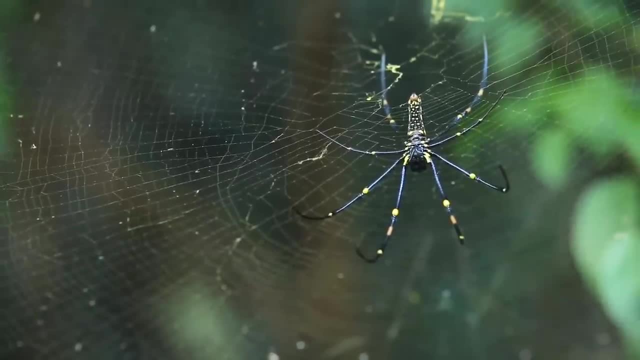 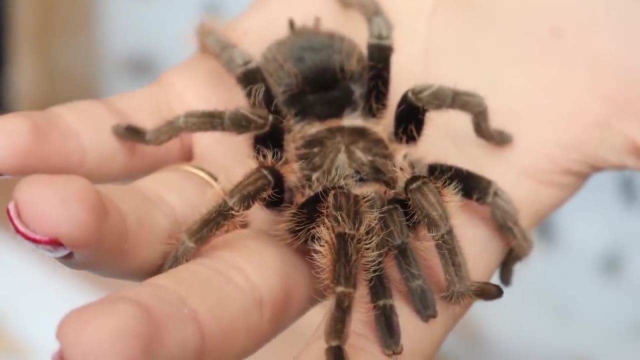 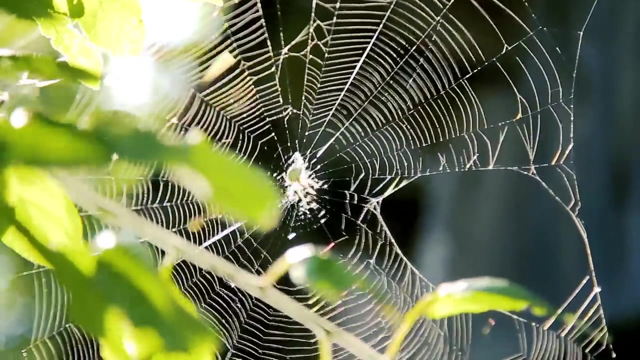 But many are not dangerous. Even though some spiders are poisonous, most are harmless to humans and animals. They are actually beneficial to our environment in several ways. For example, they help control the pest population in gardens and your homes by eating other bugs that live there. 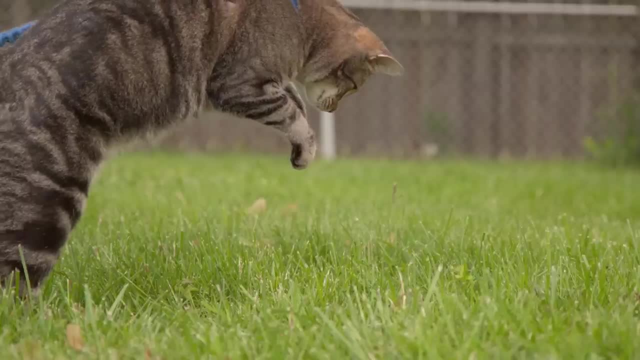 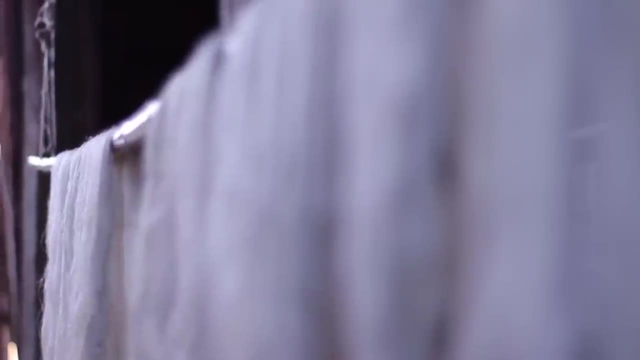 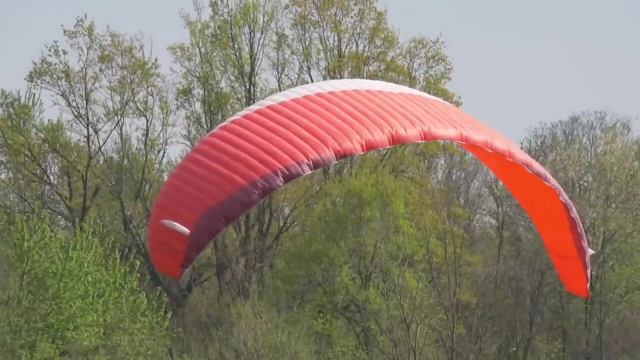 are the food for birds, reptiles and some small mammals. Some spider venom is even used for medicine. Spider silk is used to make artificial fibers like those used in bulletproof vests and parachutes. One kind of arachnid is called the harvestman, which you might know as daddy. 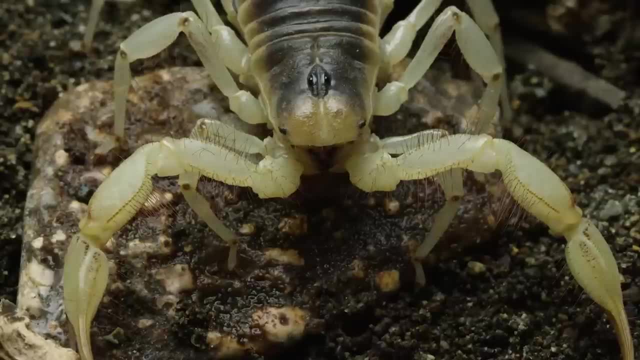 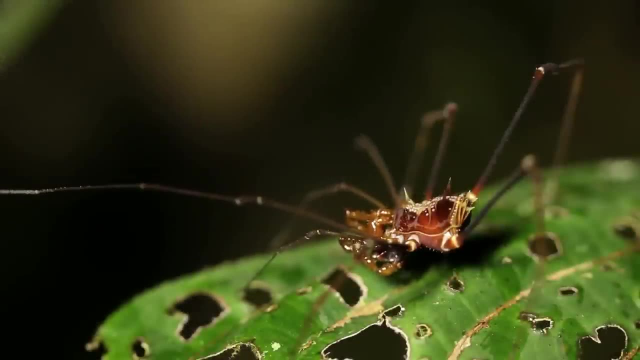 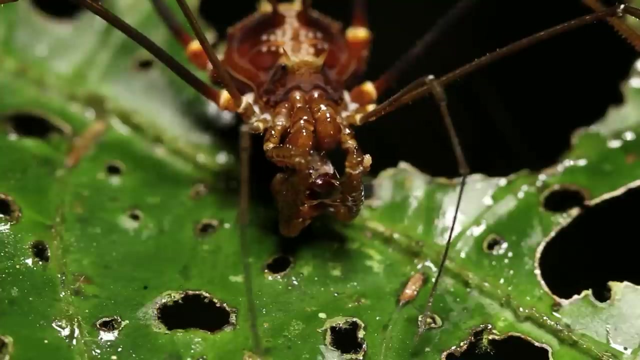 longlegs. Though they may look like a spider, they are actually more like a scorpion. They both have two body parts which are joined together as one. They do not produce venom or silk, and most daddy longlegs eat plants and small insects. Spiders have been around for a long time.